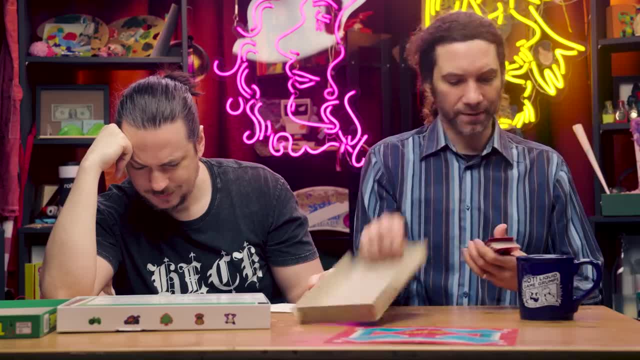 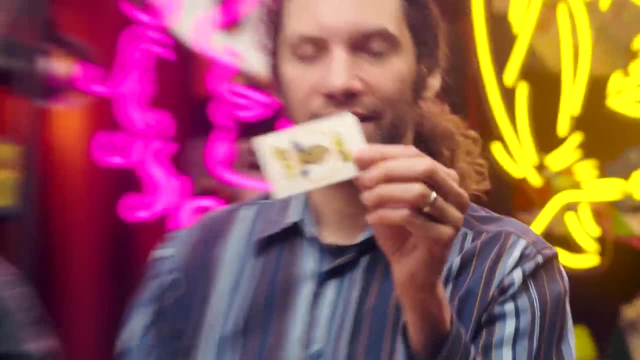 Match and collect the most cards. Let me just see what these Mr T cards are like. There's bus, There's bus, There's bus, Which is great. There's also a Mr T card. There is Mr T. He's a wild card. 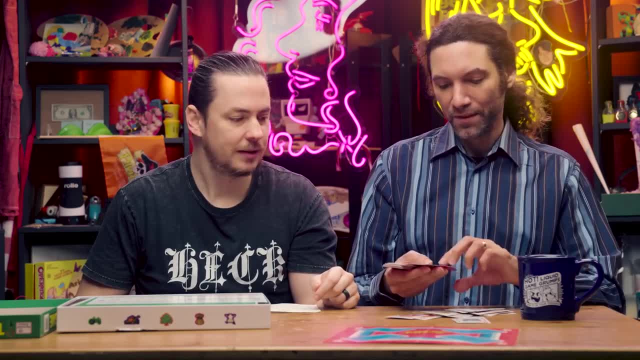 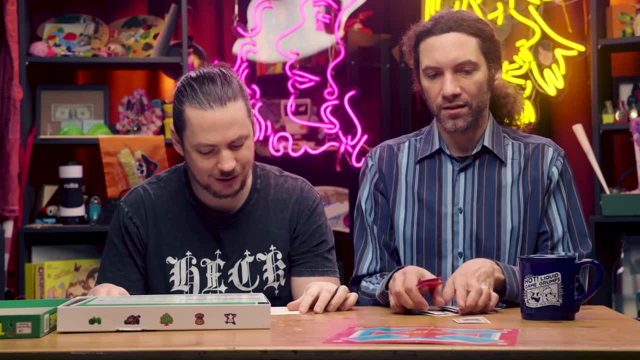 That's my card. Oh my god, It's just the same. four people over and over. No, we found Woody. Oh thank goodness. Oh my god, Woody's upside down. The object is either to be the only player to have a Mr T card showing or to have your card match another card showing for a showdown. 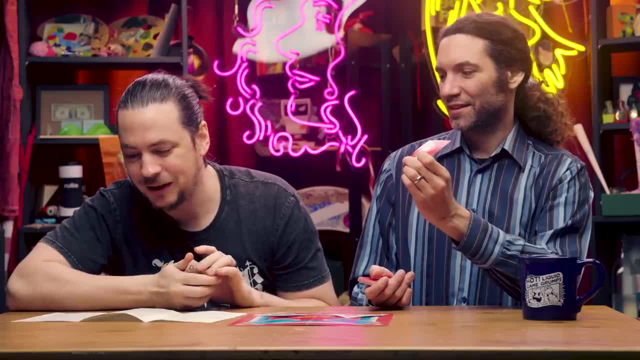 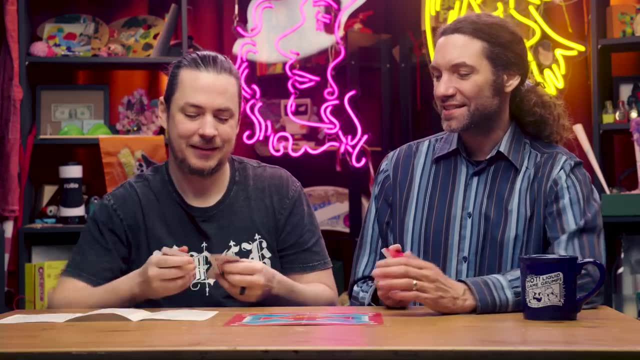 Boom, I got Kim. Jeff, This is a stalemate. No player collects the cards. Okay, I got a Mr T card F***, Which means I take all the cards. No, Really, That's that's what that means. Yeah, The T stands for thievery. Here we go And boom. 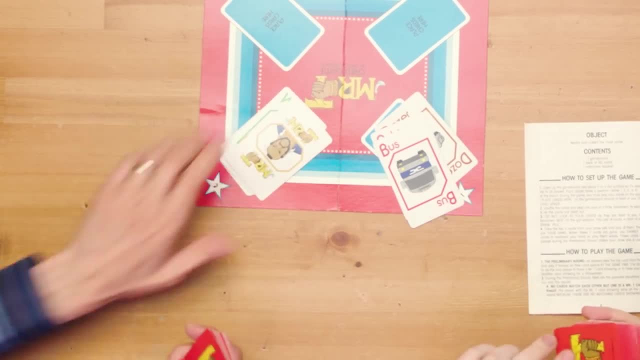 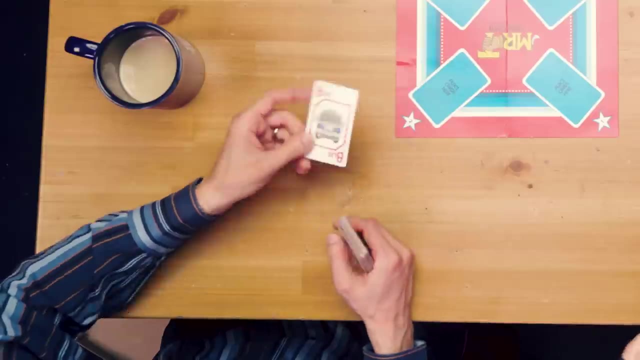 Nope, Kim Woody. Mr T, Oh, you take all the cards. F*** your bus, You suck. Sorry for cursing. Why is there a bus card? I don't know. I say we keep the bus cards from this game, Or or, Mr T? 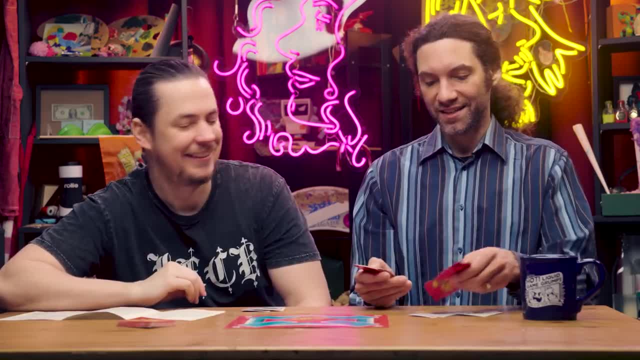 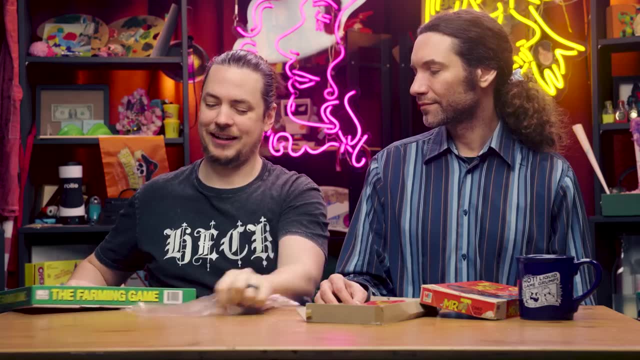 Like one, Mr T. Yes, Maybe that's like the golden ticket. Yes, a single T. The farming game- If it was called the farting game, that'd be more your style. I live the farting game where, Like, I do that risky, that risky fart, you know where it's like, I don't know what this is gonna be. 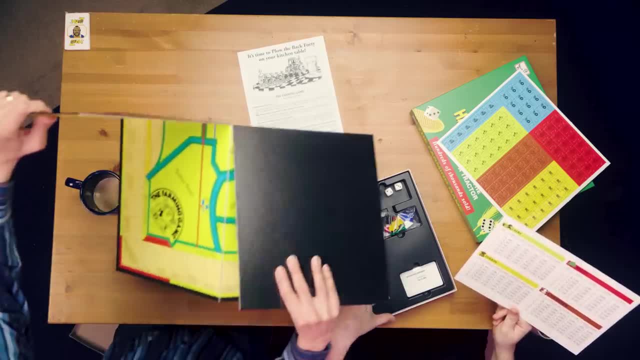 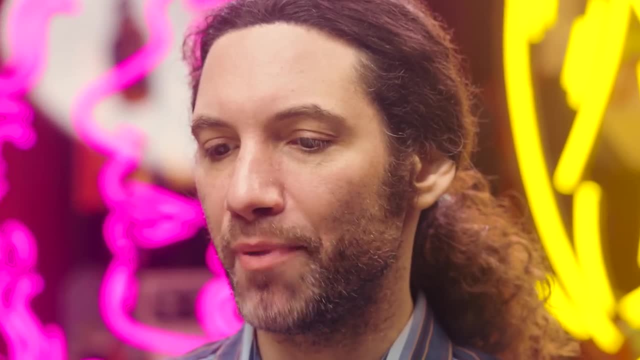 Oh my god, there's so many values. Oh, this looks. oh no, This looks complicated. Look at all these happy farmers. Look at me with my suspenders. It's time to plow the back 40 on your kitchen table. 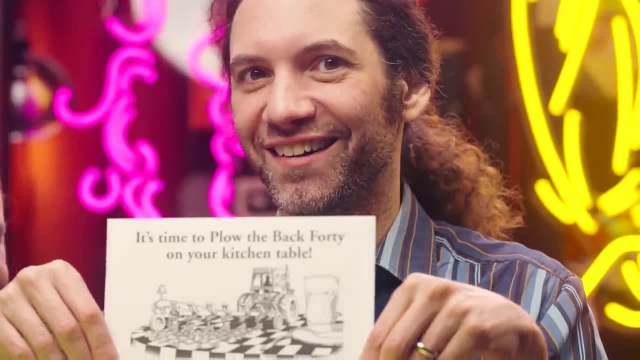 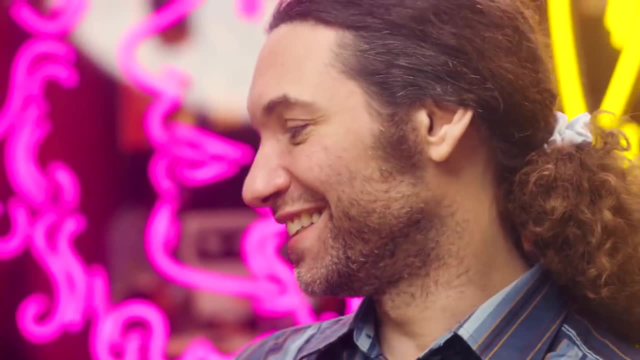 I don't, that's. that doesn't sound appropriate at all. Oh my god, Oh my god, what? Why have you done this? Wait, there's farmer's fate cards, Farmer's fate. Oh, let's keep these. 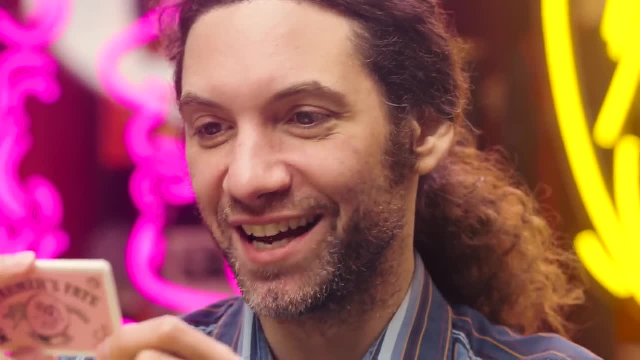 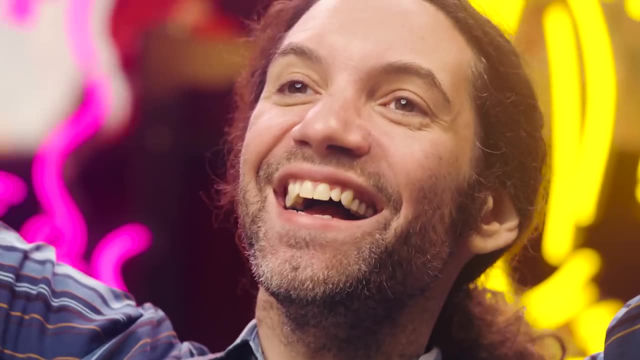 Hold on. The apple maggot fly, cousin of the dreaded med fly, is found in an insect trap in your orchard. Your orchard is quarantined and you lose a lucrative export contract. Oh my god, Yay, This was made by an actual farmer who went through some 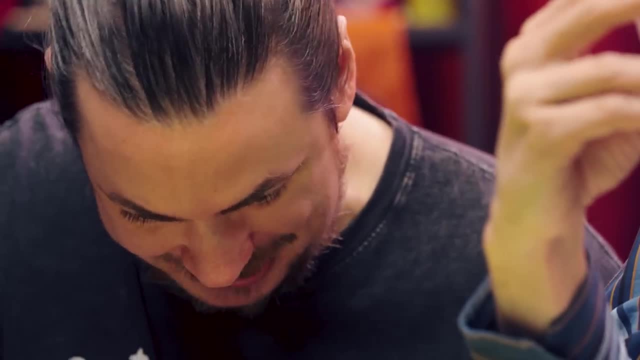 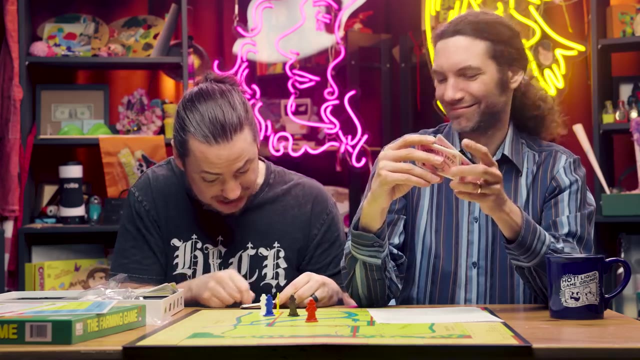 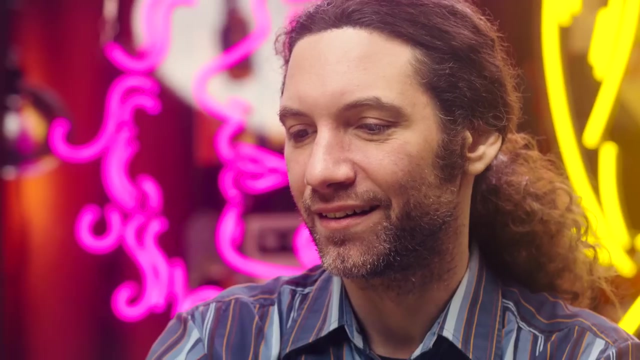 Oh yes, A leaking electrical motor and feed mill contaminates your load of feed with PCB. State Ag Inspector requires you to slaughter cows on your farm With no reimbursement. It's a terrible farmer's fate. Well, we're keeping these. 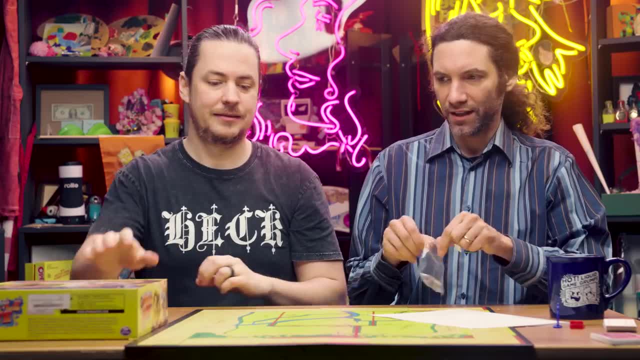 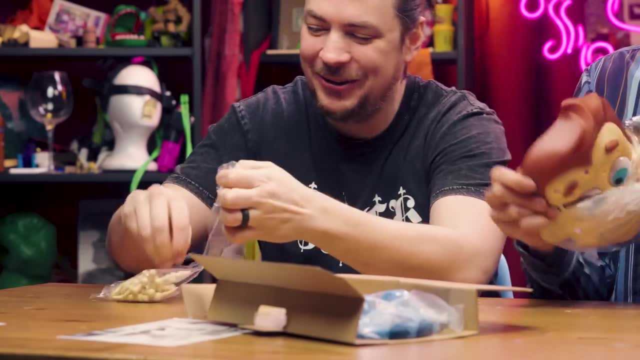 Yeah, we're keeping the farmer's fate. This is a good one, Hold, hold, I haven't even gotten the farmers back in there. That's disgusting. It's pimple peat, The pressure-packed pimple popping game. Look at this thing. 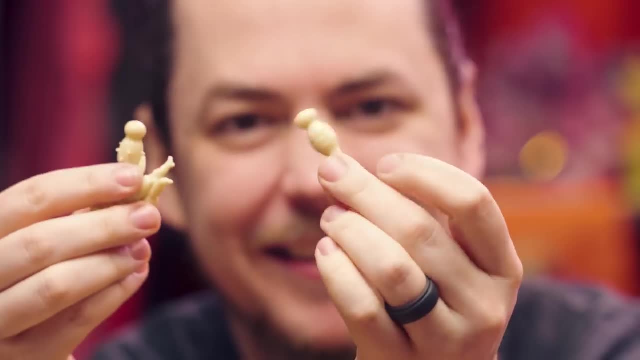 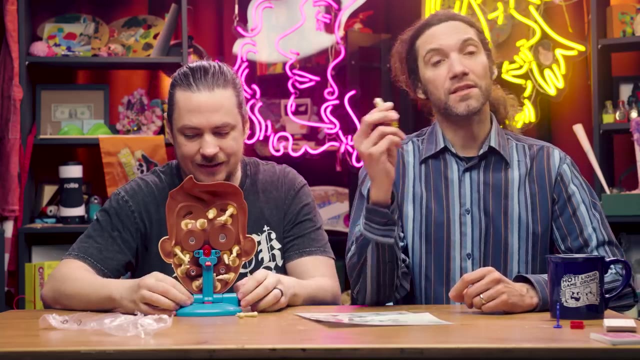 There's gooey pimple pieces that look like little spermies. Just put these little pimples in. Oh, they feel terrible. They're ooey gooey. Alright, How's that? This is the Mega-Zit plunger. Draw the water to the fill line and then load it up in the little spot. 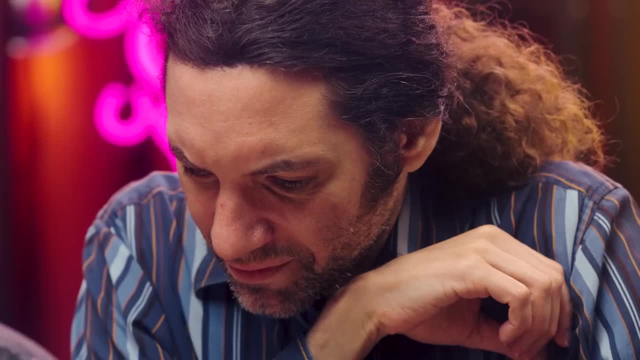 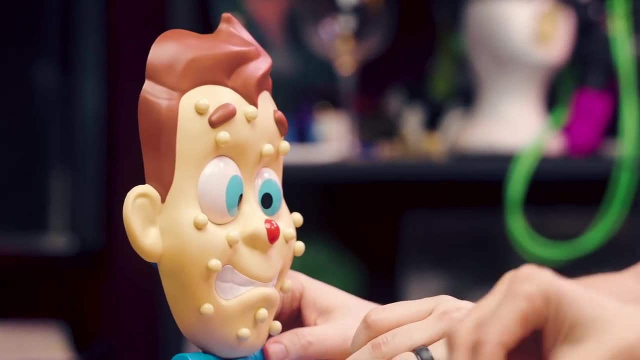 The Mega-Zit is ready for play. Too much movement may cause it to burst. Oh, I see, It's just very sensitive. You gotta get it to spray at us. Oh, okay, You know. so maybe like this, Yeah, sure. 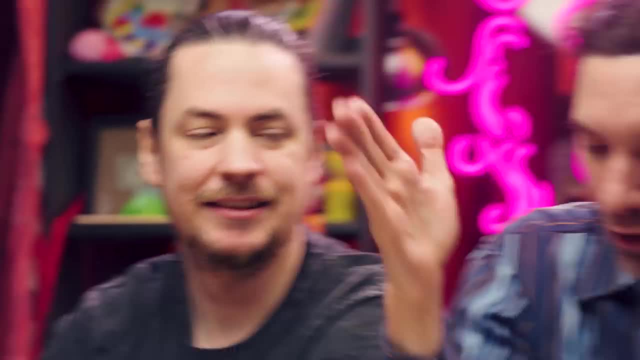 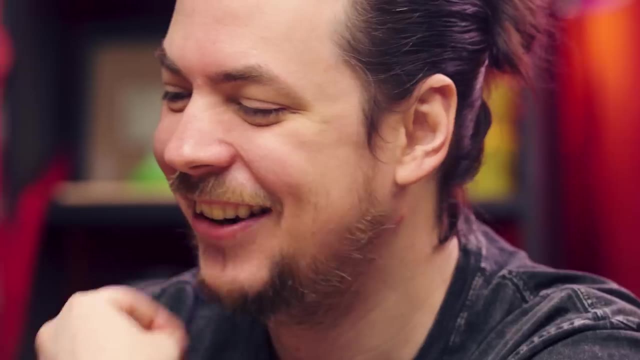 Pop the pimples without bursting the Mega-Zit. If you burst the Mega-Zit, you forfeit the pimple and get no pimple points for that round. Clean yourself off. Alright. well, let's go Forehead, okay. 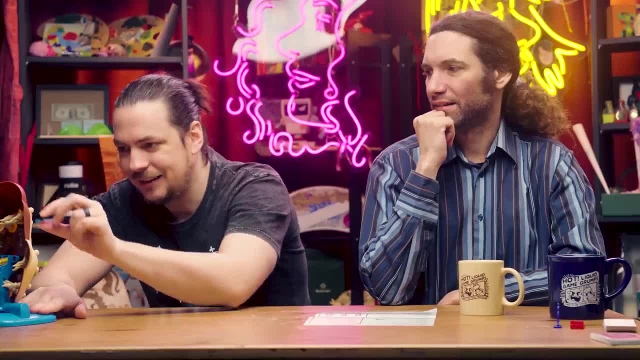 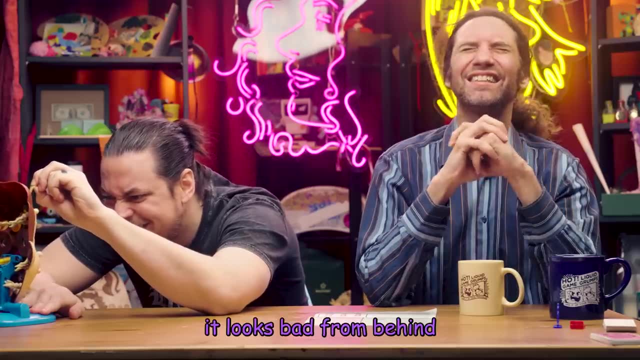 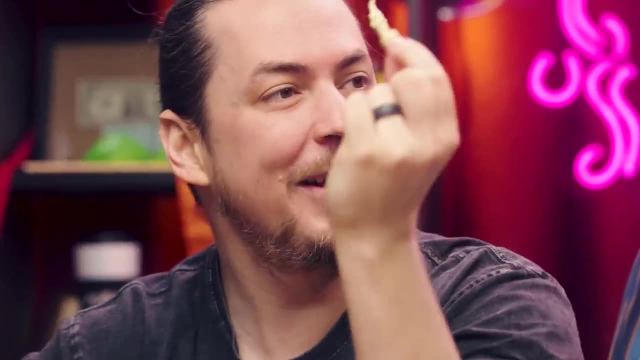 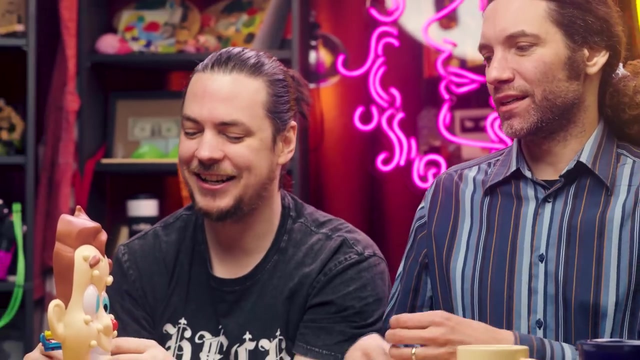 So you use one hand to hold the base and then you pull. It looks bad from behind. It looks bad from all angles. Yeah, I got three points from that one baby. Now it's your turn to spin. Right cheek, Right cheek. 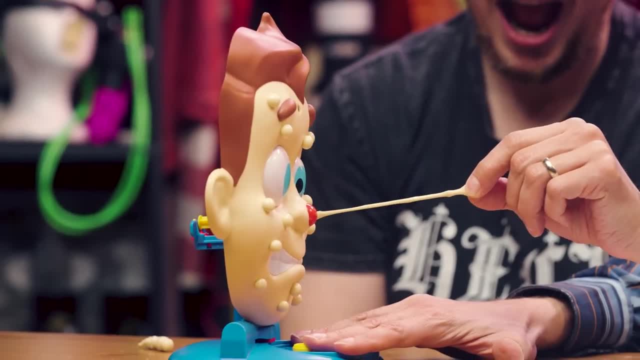 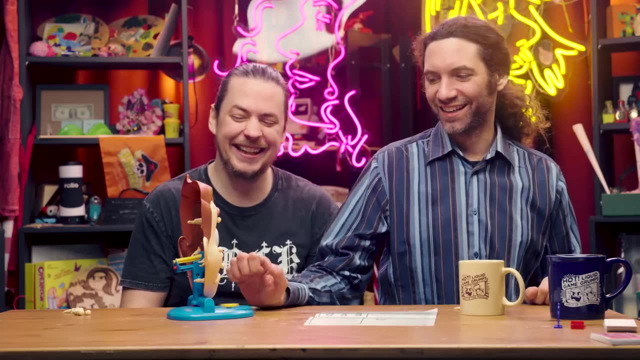 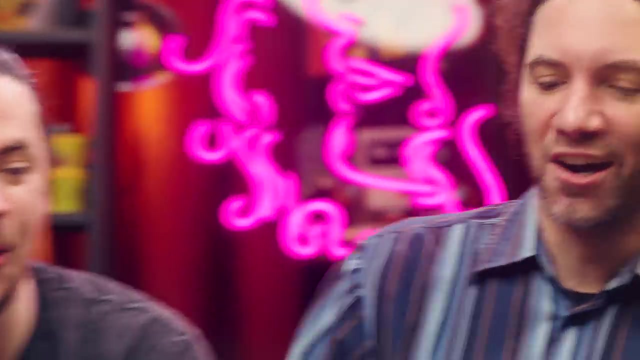 Oh, that one was easy. Oh Oh, How many did you get? I hate it. How would I know Two. It's kind of fun. The premise is f***ing gross, though. Oh Yay, You won. 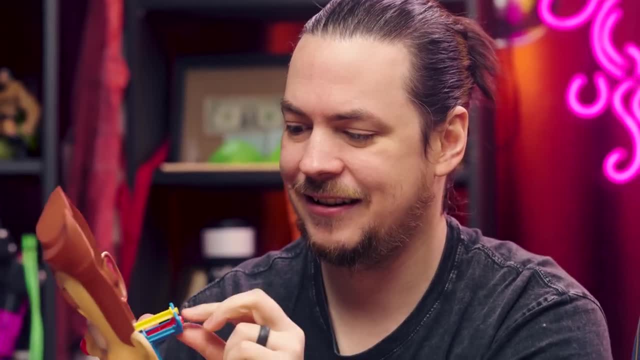 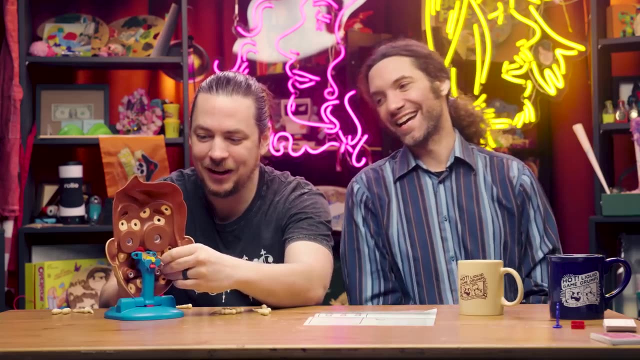 I won. I got nine points. Did we do this wrong? Did I, like You, forgot to take the safety off? Oh, Ew, No, we're not doing it again. Hold on, I just wanted to try once. 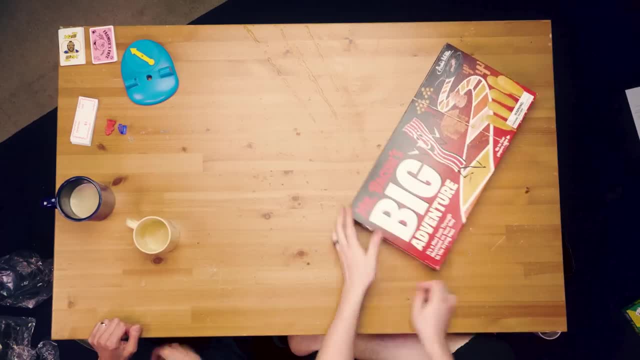 Alright. so what do you want to keep from this game? Nothing, Ah, That was vile. Mr Bacon's Big Adventure: Whoa, Oh my god, It's a mad dash through Meatland on your way to the frying pan. 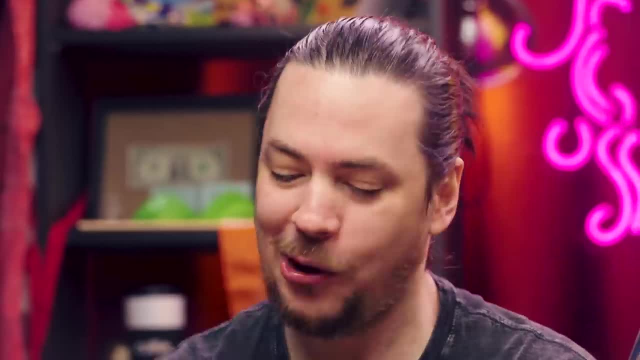 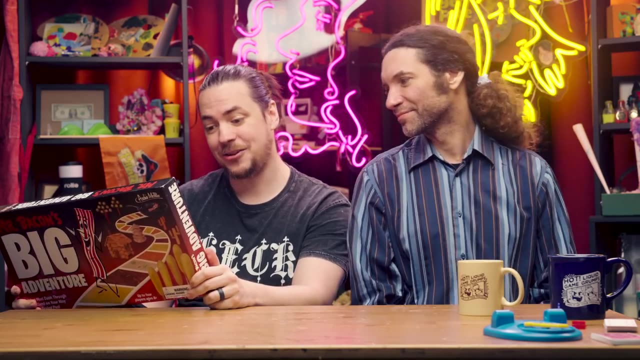 Okay, we immediately went from my least favorite to my most favorite. Look at the corn dog, cactuses, Cacti, Wow. Join Mr Bacon on a mouth-watering mosey through Meatland. On your journey, you'll have to navigate your way through the Mustard Marsh. 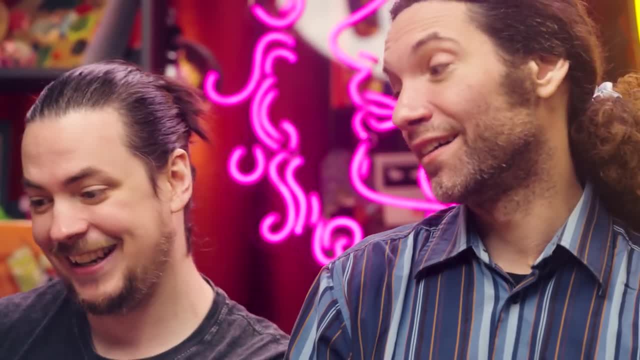 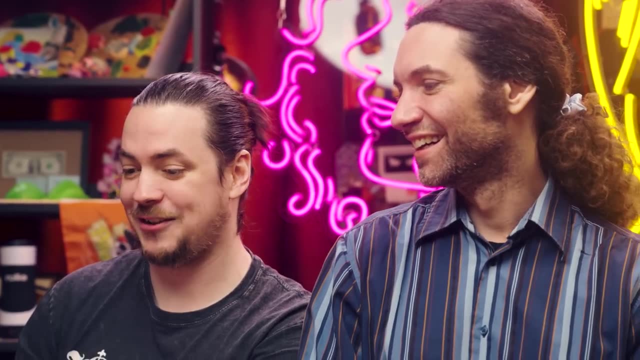 Cross the eerie expanse of the Wiener Wasteland, Oh, And sail on the Sausage Sea. Wiener Wasteland's gonna be the new name of my Wi-Fi If you make it past the deceptive detour of Vegan Alley. 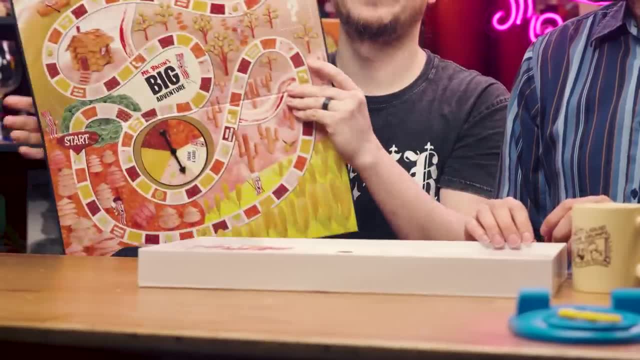 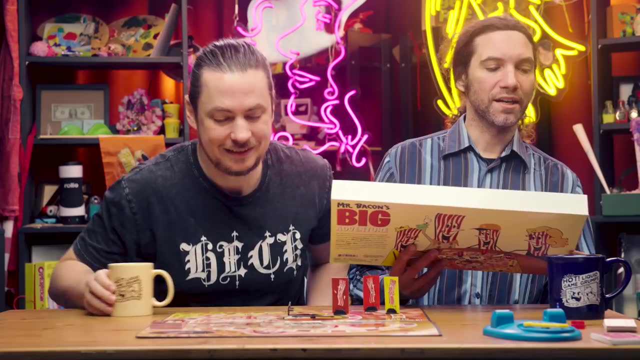 Oh, my god, Look at that, Look at that board. Mm-mm-mm. Hey kids, Remember, cheaters never win and winners prefer meat. The object is to be the first strip of bacon to the frying pan. Ooh. 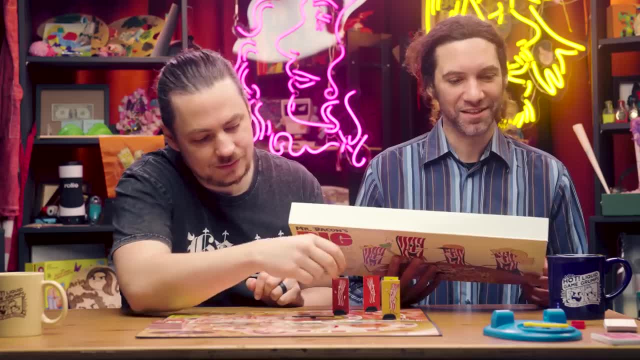 God, if I was a sentient pig that could understand this, I'd be happy. I'd be so pissed off. Spin the spinner and move to the color that the spinner points to Just make it to the end. I mean, it's like the easiest game in the world. 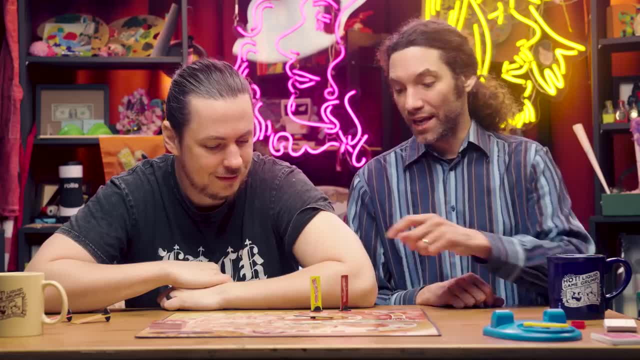 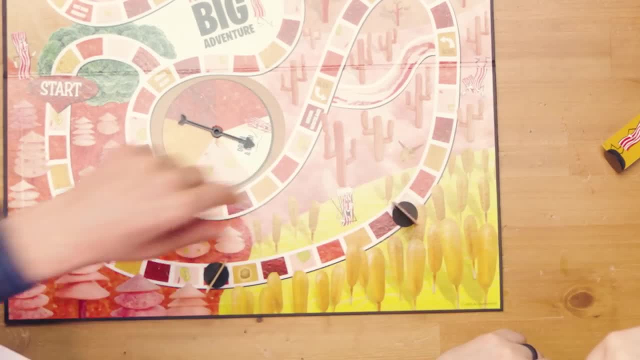 All right, go ahead and spin All right Pimento loaf. Okay, draw a card. Oh, you can draw a card. All right, here we go. Move any player to the Mustard Marsh. Oh, Oh, Oh. 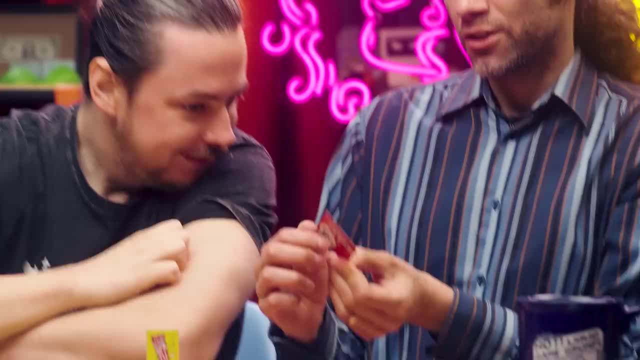 Oh, See you in hell. You're an asshole Meatball. you gotta draw a card. Oh, he gets to draw a card. Go bang out in the hot dog hideout. Go hang out in the hot dog hideout, Sorry. 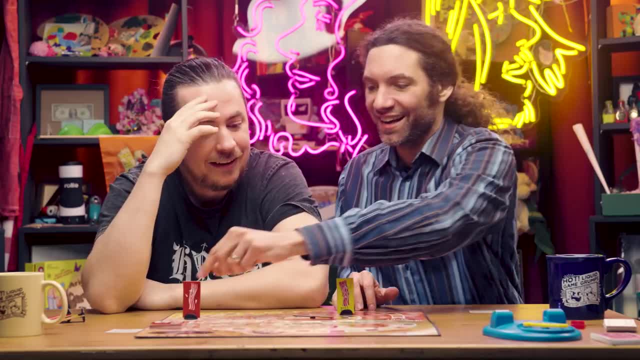 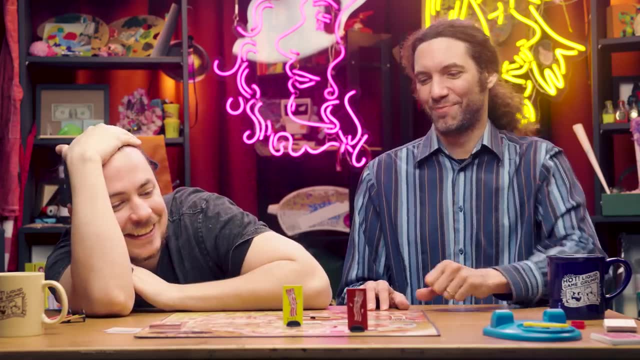 I thought it said: bang out too, Yeah, yeah, Oh, my god, that's so far ahead. Hell yeah, Hot dog hideout. Stop winning. Stop winning. You hate losing. Stop Even at Mr Bacon's Big Adventure. 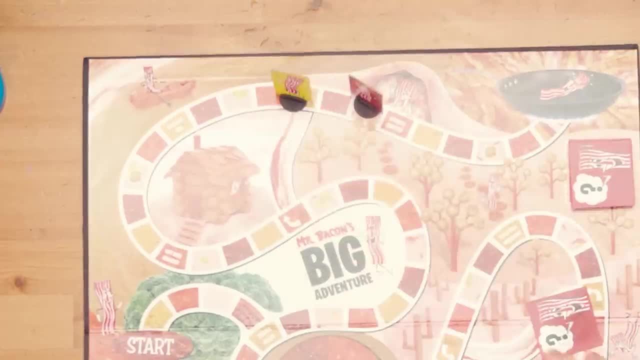 Move forward or backward to the nearest bacon slide. Yeah, Oh man, It's gonna come right down to it. It's so exciting, Oh Gristle Grotto, Oh, that's a thing, That's a special thing. 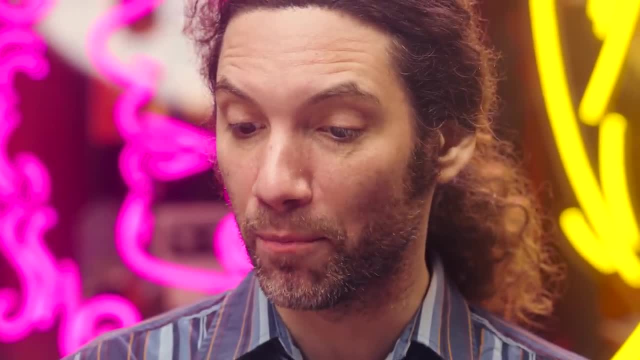 Is it? Yeah, If you land on the Gristle Grotto space, you are stuck there until the spinner points at the corn dog color on your turn. I totally got screwed. Ooh, draw a card, Go directly to Gristle Grotto. 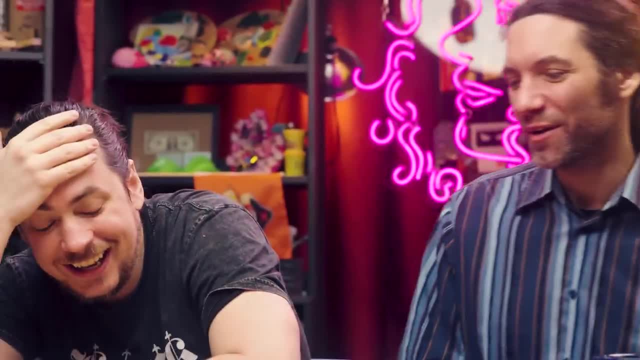 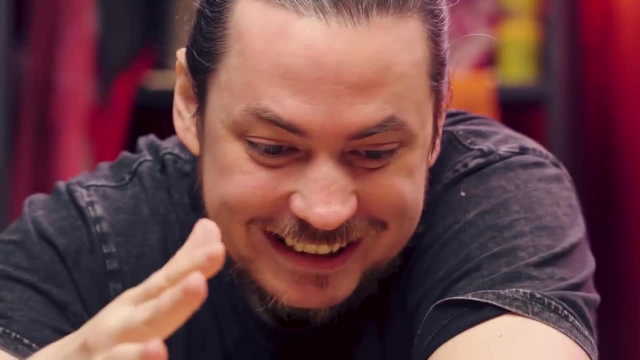 Yay, What the Hey dude. Now we have to spin until we point at the corn dog. This is actually a shockingly intense game. Gristle Grotto, you nightmare. I'm stuck forever in Gristle Grotto. 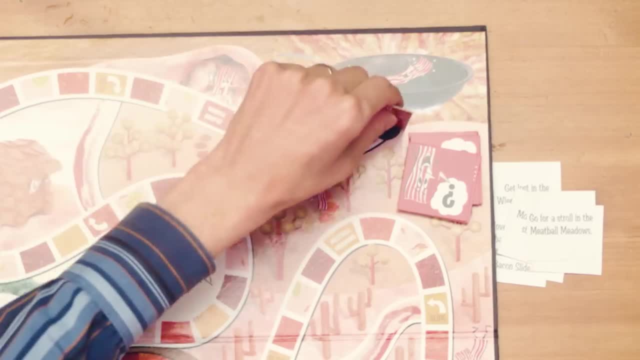 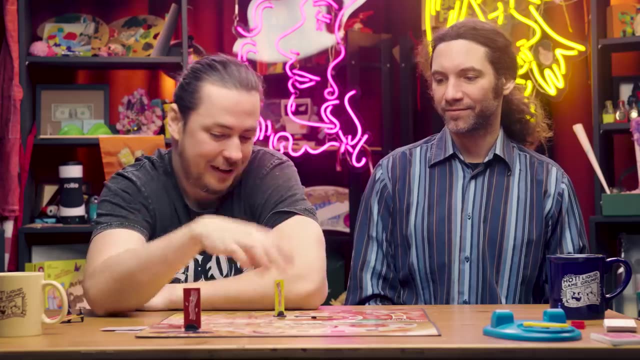 Yeah, Oh no, I think I did it. Yeah, I think you did it. I think I did it, I made it. I am the bacon that gets fried and eaten. Well, good, I'm alive. I can just go back home and my wife. 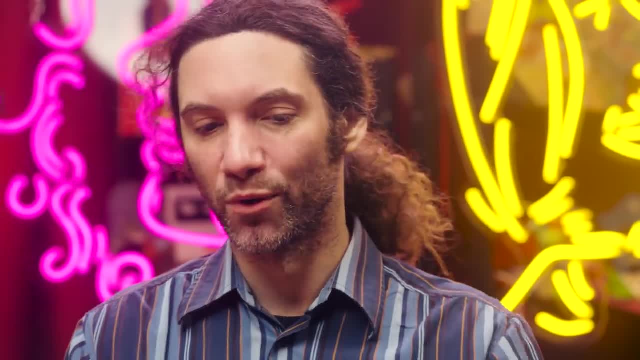 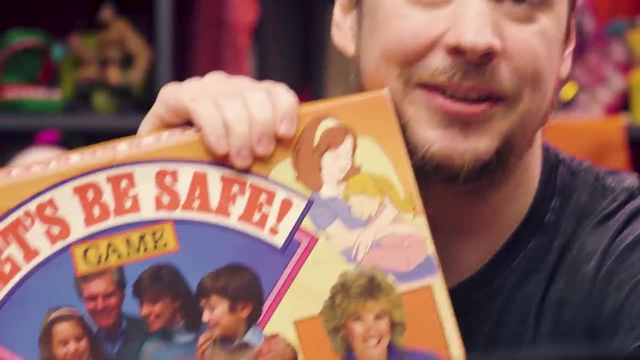 Maybe this is the one where we keep the board. Yeah, it's a good looking board. Yeah, Ah, It hurts. Let's be safe. The fun way to alert your child to dangers at home and in the neighborhood. Don't talk to Carl. 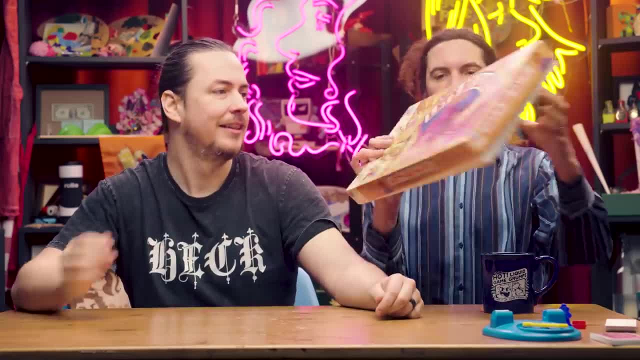 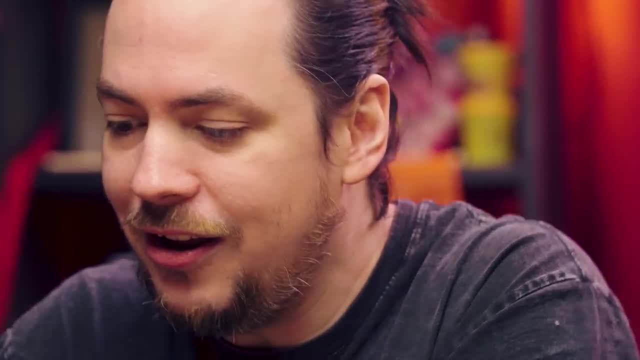 Unfortunately, Carl, is this man posing as their dad. Any time you land on a yellow space, draw a situation card. Then try to match the situation card with one of your solution cards. Sounds great, Go for it, Mm-hmm. 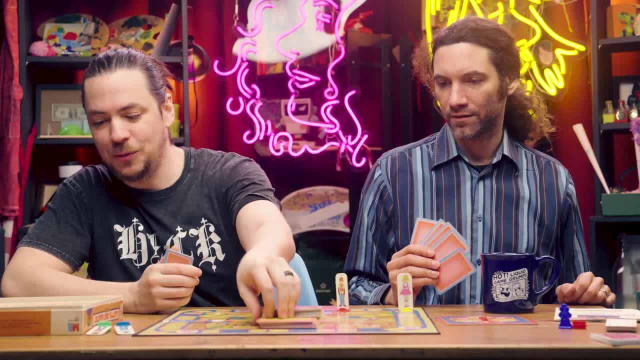 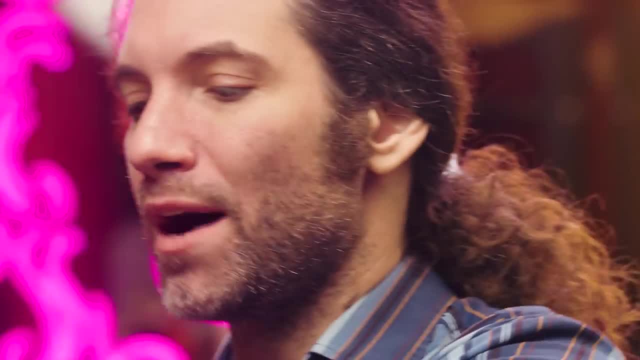 Four. One, two, three, four. Oh, We draw a situation card. Okay, A stranger comes to your door. I'm going to play. don't touch food that you find. Ask mom or dad. Boom Bitch, Yo, that's like a trump card. 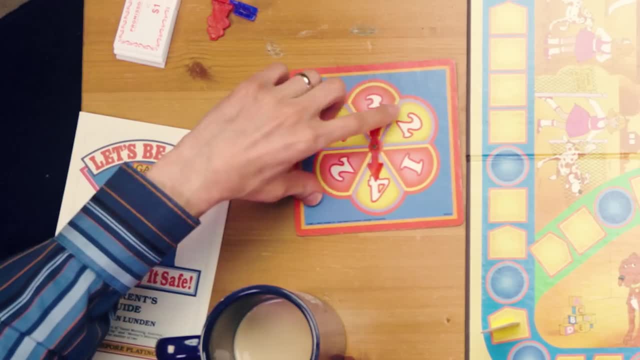 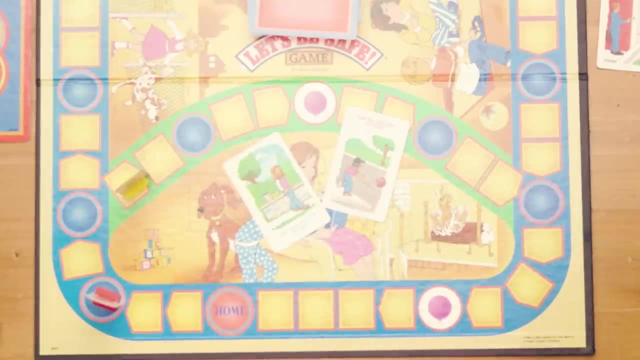 I know, I know That's a powerful card. Oh, This is fun. Being safe is fun. Your ball goes into the street. Uh-huh, Don't touch that food you find. How about ask a grown up to get your ball? 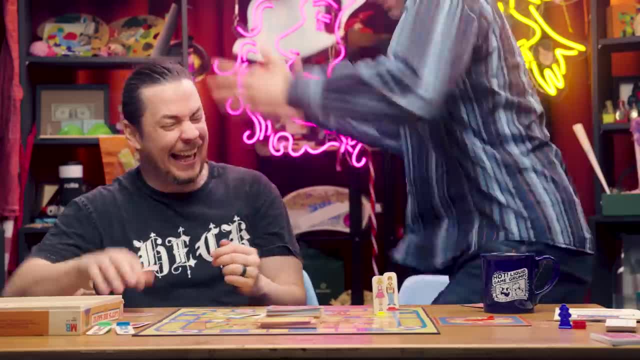 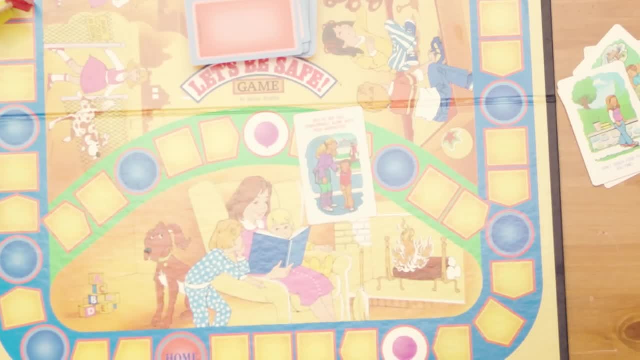 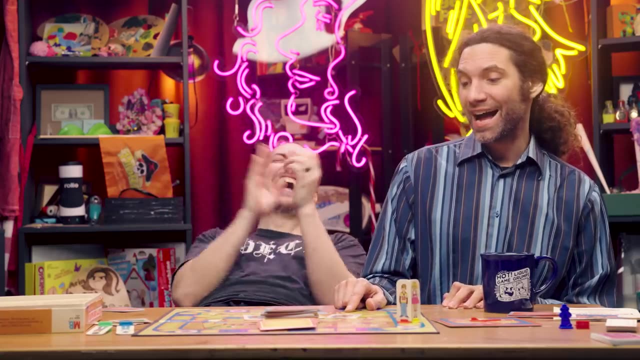 Oh my god. Oh Okay, Go ahead. It's you. Oh, You do not feel comfortable alone with your babysitter. Don't matter who the babysitter is. No, I have a match. I have a match. It's who calls it first? 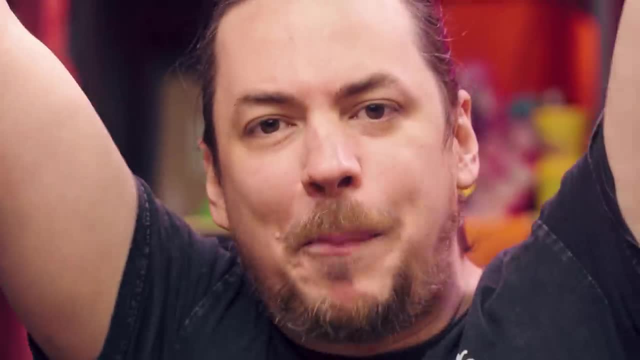 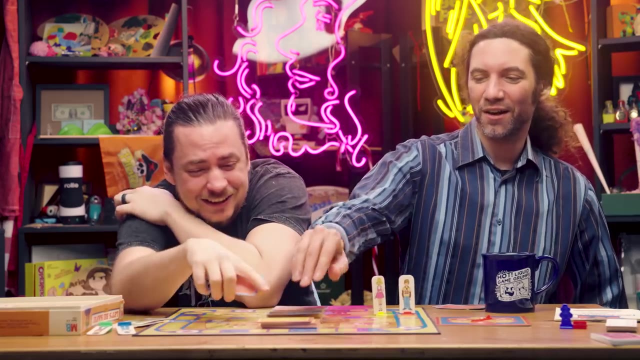 No, it's not. Yeah, I don't feel comfortable babysitter. I didn't feel comfortable around the babysitter either. frankly, I did Two ahead. It's a new, That's a solution, I'm sorry. I'm sorry. 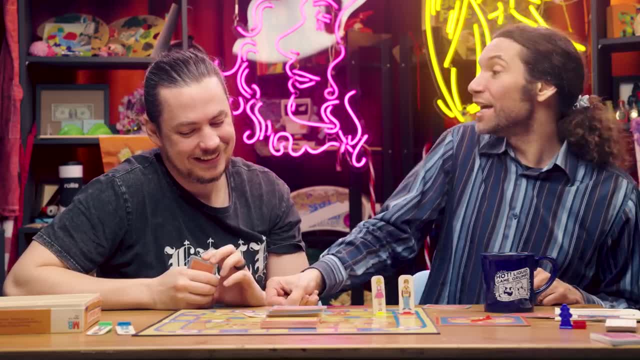 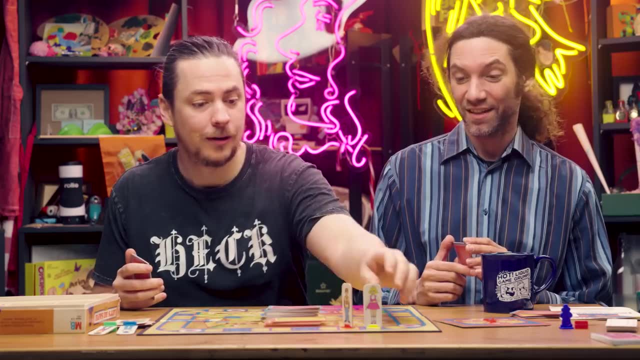 Your little sister wants to play with you. How about find something you could teach her? It'll be fun. Yeah, How are you so amazing at this? Four, That's a, That's a huge thing. Four. Sorry, I knocked you over dimwit. 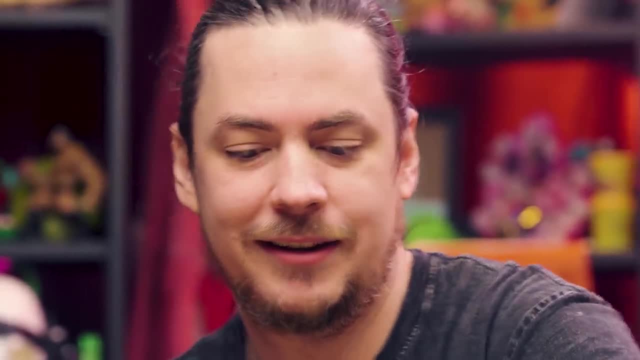 A grown up is holding you and makes you feel uncomfortable. Yeah Well, if you feel uncomfortable, you can say: no, Oh, Oh, Oh Oh, I can't believe this game is super fun. No, You made it home. 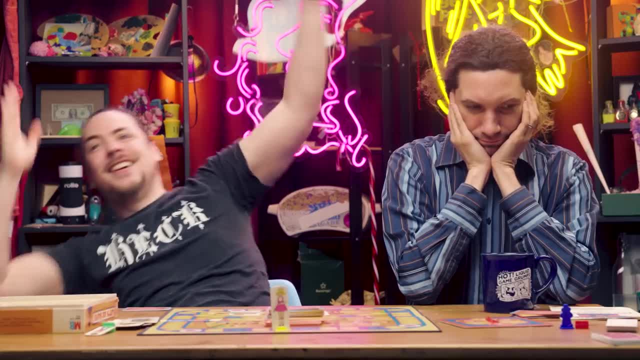 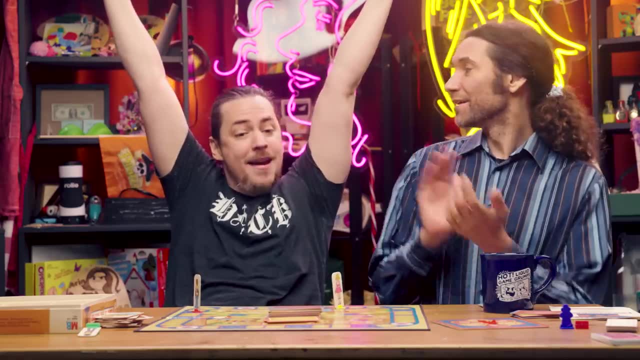 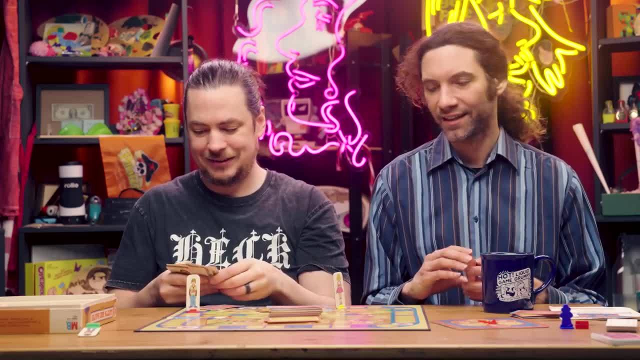 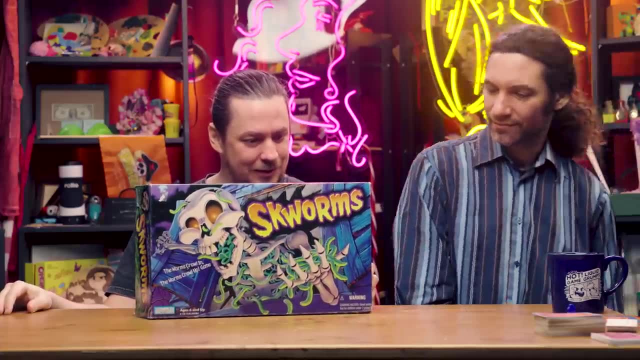 So what should we keep from this one? Dan, The solution cards. We should keep the solution cards. Yeah, Yeah, Okay, Squirms- Whoa dude, Look at this. This is bizarre. Can you be the first to get all your squirmy worms up the skeleton's bones and into his? 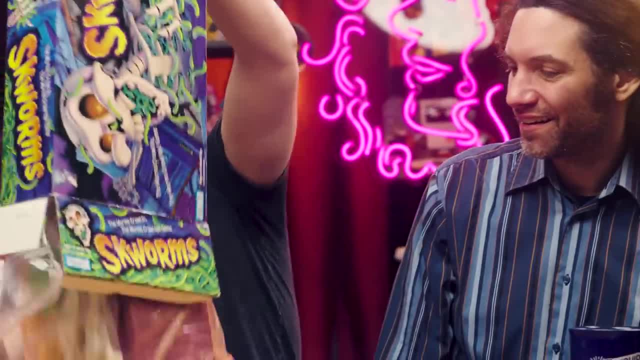 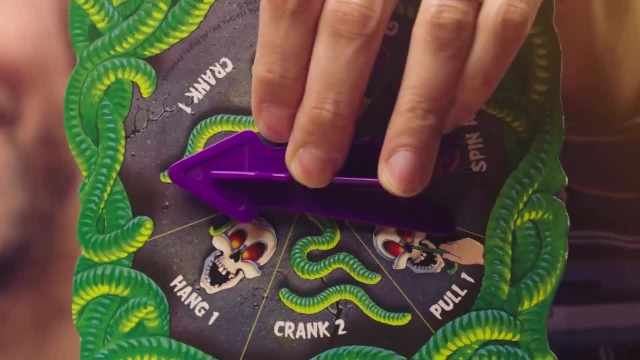 skull. All right, squirms, Uh-oh, Listen to that. Ooh You ready for these directions, Arin? Yeah, Hang one, crank two, pull one. Yeah, Sorry, I just hung one and cranked two. 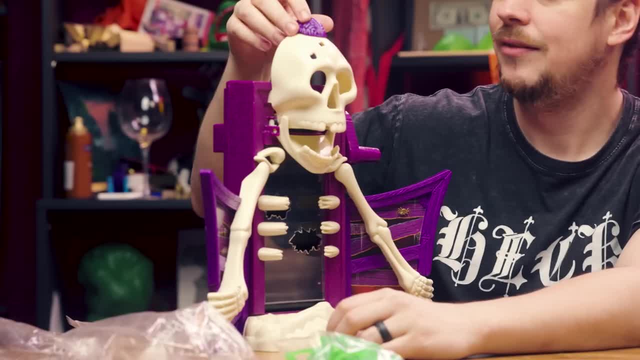 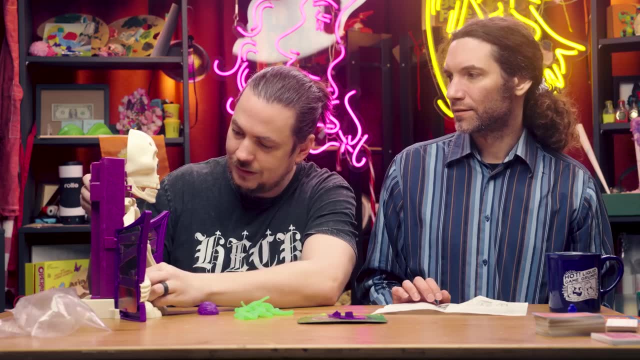 Where does Brain go? Mazel tov, It's his bone. mitzvah Crank two Oh, Oh, Oh, Oh Oh. This game is dumb. Look at him squirm up. That's cute Oh. 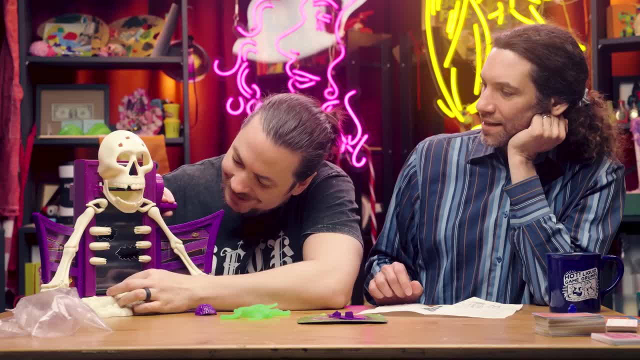 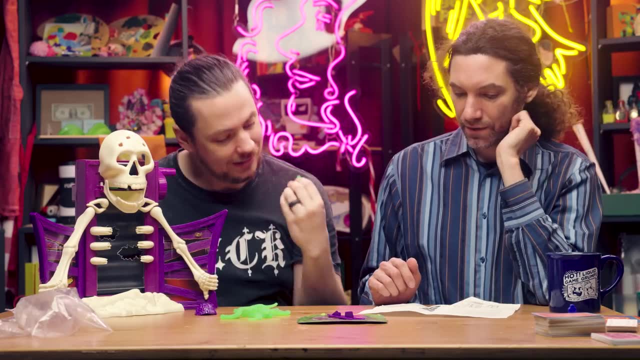 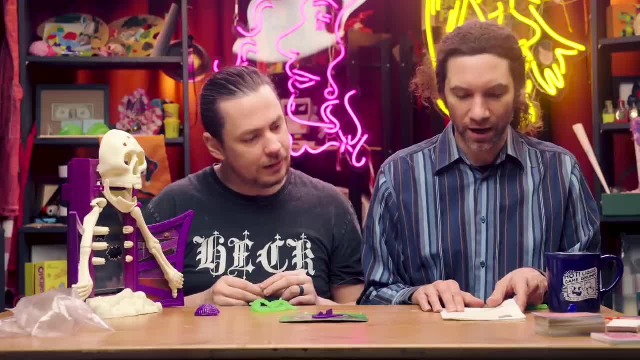 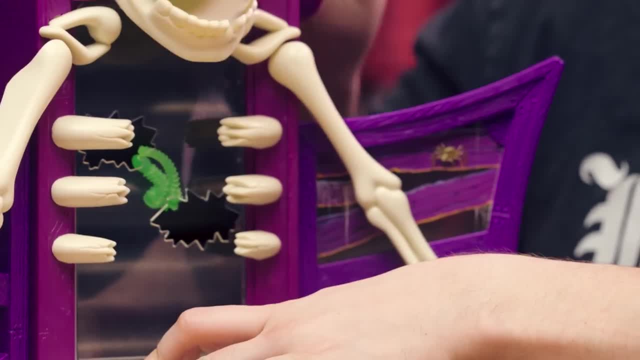 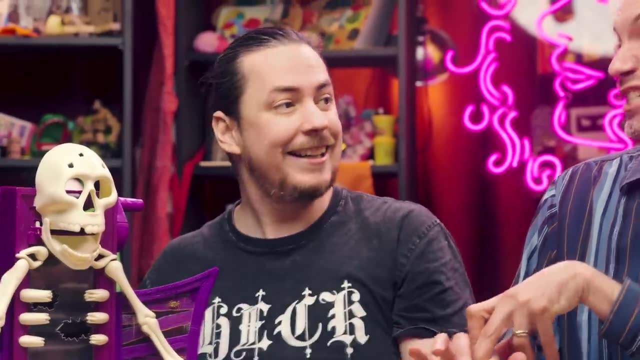 No, I give you the brain. So you have the brain, Because you got to give one, though You did not Crank one. Oh Oh Yeah, Put that worm up and Oh Holy Snicked. 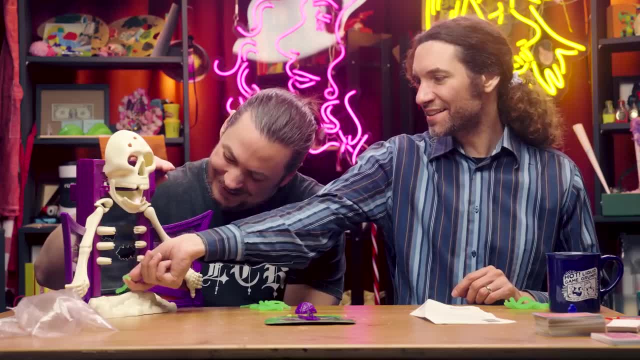 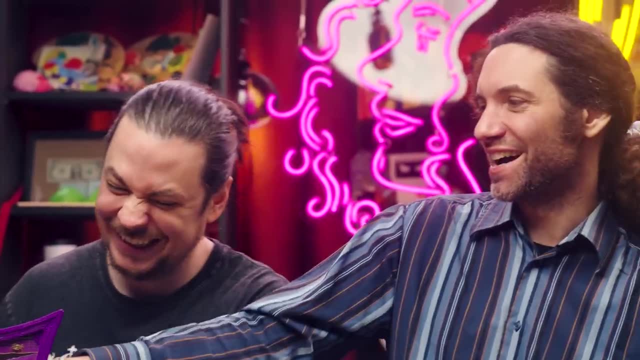 It's like the world's lamest Wolverine costume. Mom, Dad, I hate this. There's always next Christmas. Nom, nom, nom, nom. You can't violently crank it until it spits it out. Give it to you, you freak. 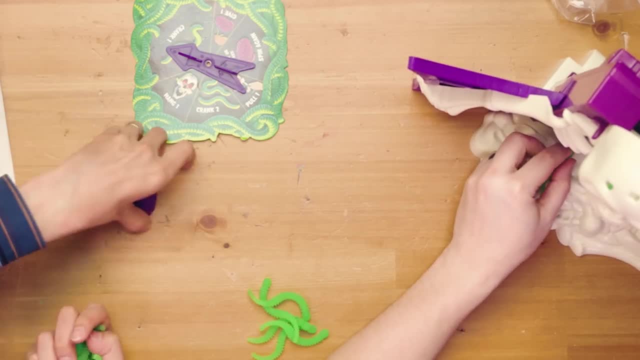 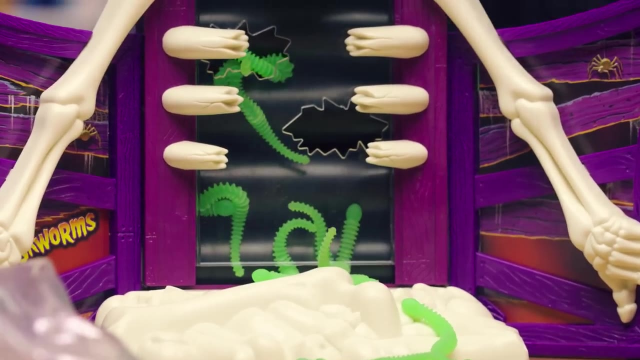 Can we stop playing this? It's never gonna end. Okay, well, we'll just. we'll take the brain. Just put all the worms in at once. Look at all the worms go. Did you do that to the tune of Bullet With Butterfly Wings. 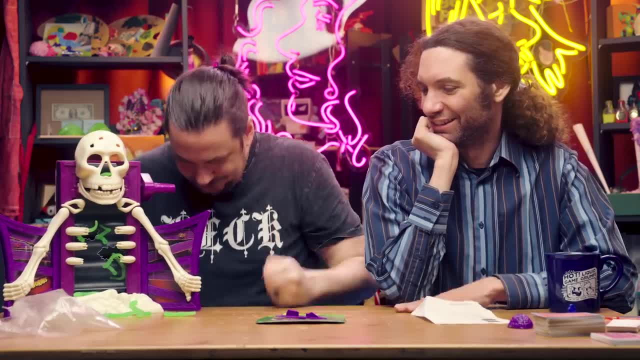 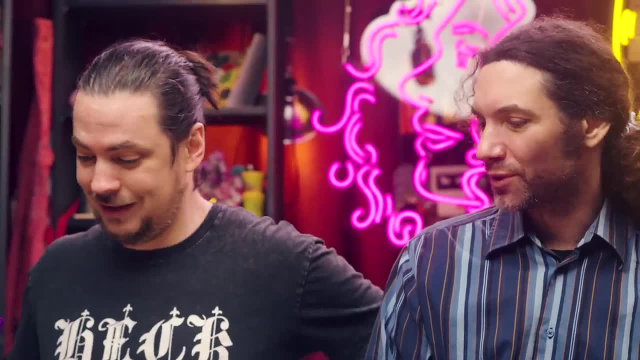 The worm is a vampire Sent to cry a yank. I love how he's like. no, don't. Great game, great game, Awesome Cootie, The original Cootie, A preschool game toy for two to four players. 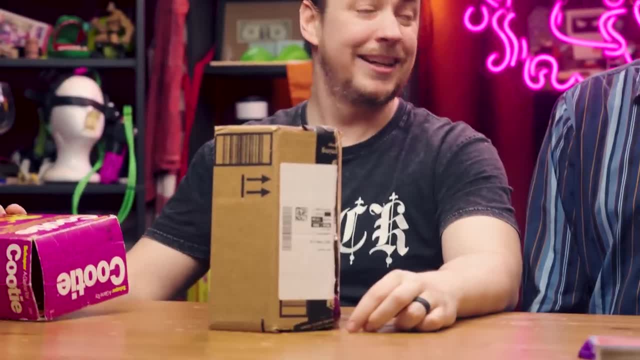 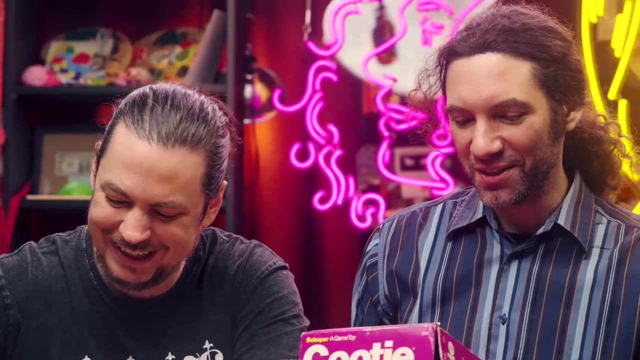 and you don't need reading skills. I got a package. Yeah, wow, Build a Cootie Bug by rolling the Cootie Cube or the dice to collect the parts you need: Body, head, ears, eyes, tongue and legs. 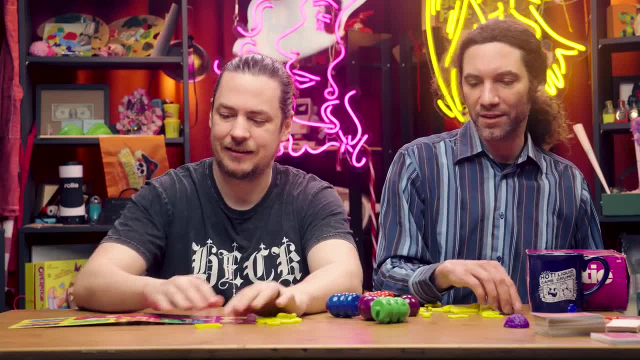 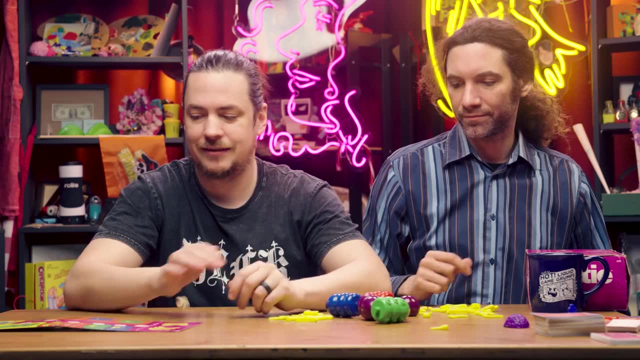 So I guess we start from nothing and then we roll and start collecting. I think that's right. Five: You get a tongue. Okay, It's this, Thank you. Six: I get a leg. This kind of is fun. Two: 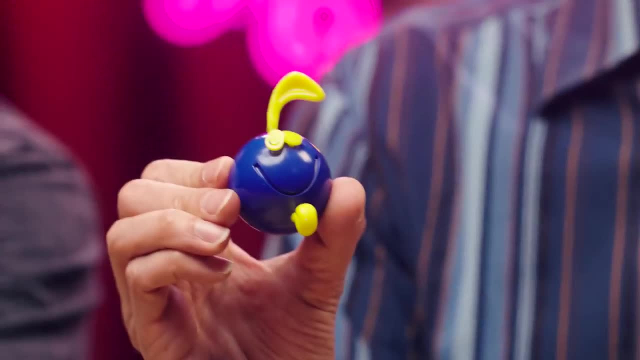 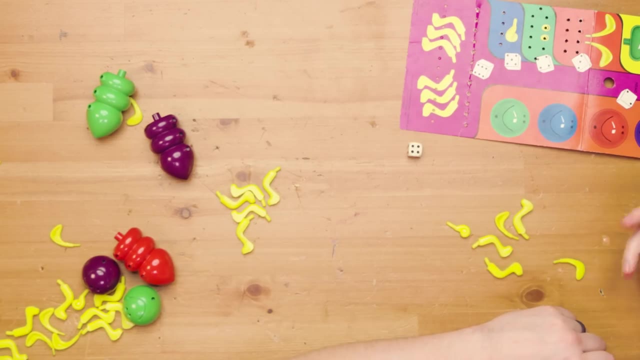 A head A head. I'll take the blue. Look at my Cootie Roll. damn you roll. Okay, sorry, No, Yes, I get the body of my schwoz Oh eye. Yeah, that's good. 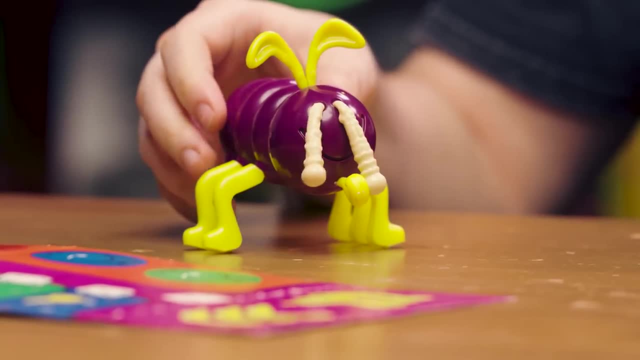 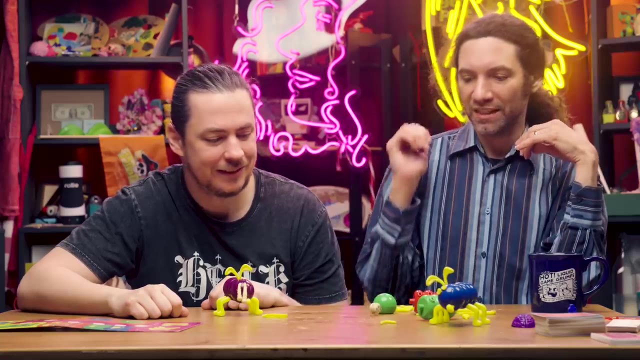 There's no eyes. We're out of eyes. Oh, your Cootie is a monstrosity. Get the hell away from me. Oh my god, we're both one away. I'm one away from a completed Cootie. 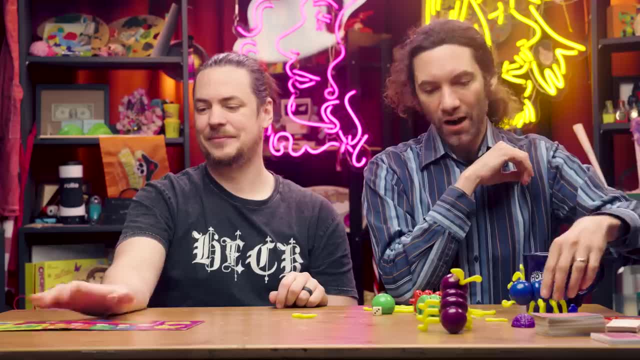 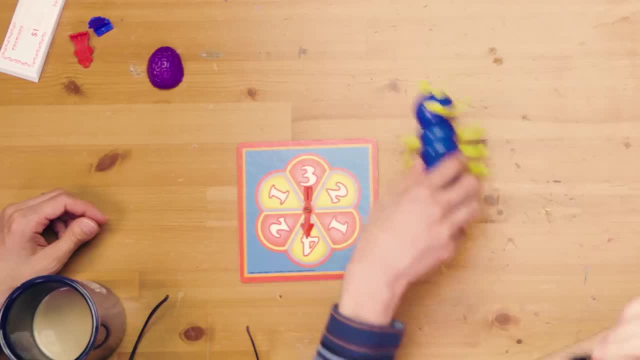 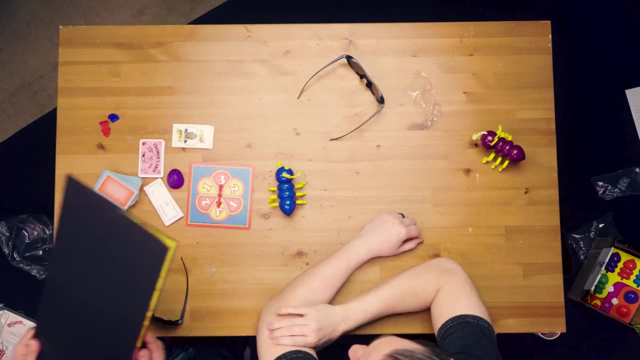 Yeah, All right, Keep the Cootie. Do you want to keep yours too? Yeah, I hate it. We have all our pieces here, Our Cooties, a little brain, solution cards. Solution cards, The farmer's fate, Mr T cards and the bacon board. 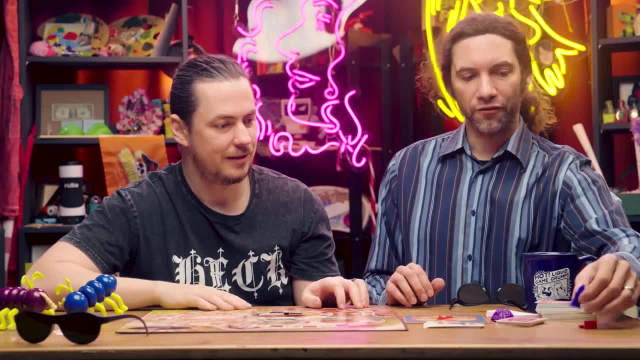 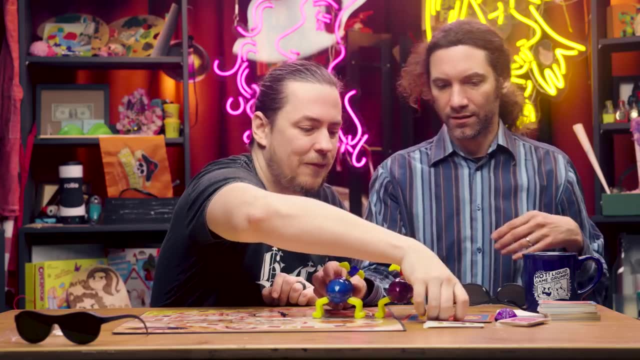 Oh, the bacon board. yeah, Our pieces should be our farmers riding our Cooties. Okay, here's yours. All right, I'm just going to wedge them. We'll roll to see how far we go. Okay, that's spinning. 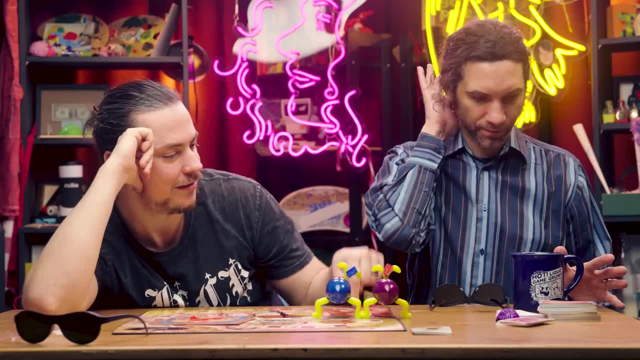 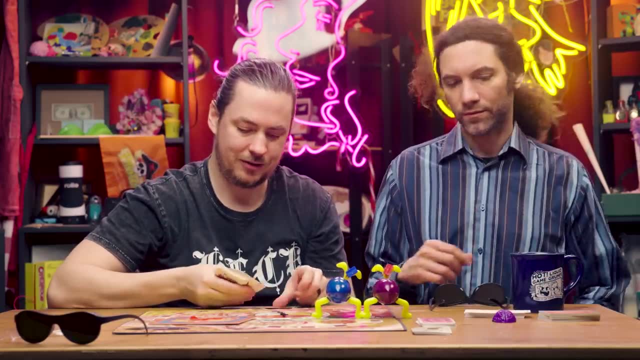 Mr T cards. Mm-hmm, We're dark, red and farmer's fate cards are yellow. and then we each have a hand of seven solution cards. Okay, At the end of each turn, you pull a farmer's fate card. 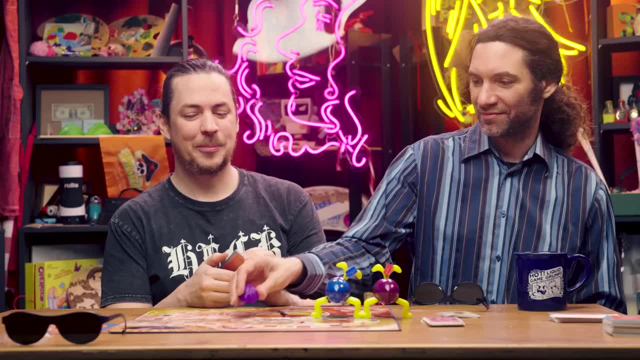 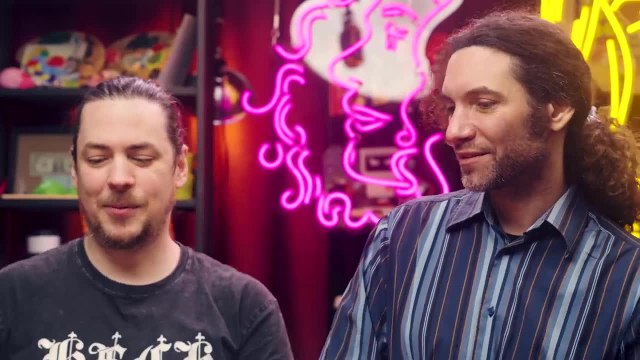 and try to solve it with the solutions that we have, Right? Well, the brain should be a piece. Okay, It's like if I have the brain then I can narrowly avoid the bus. So you get the brain by getting the draw card. 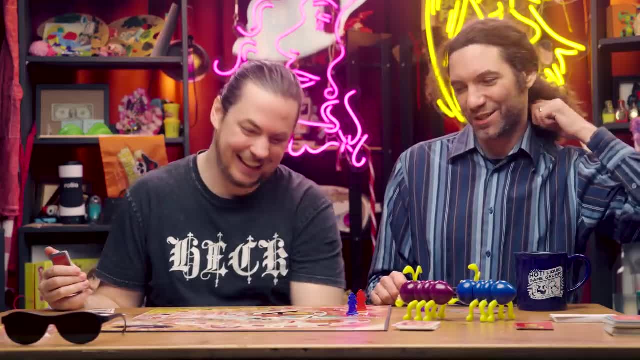 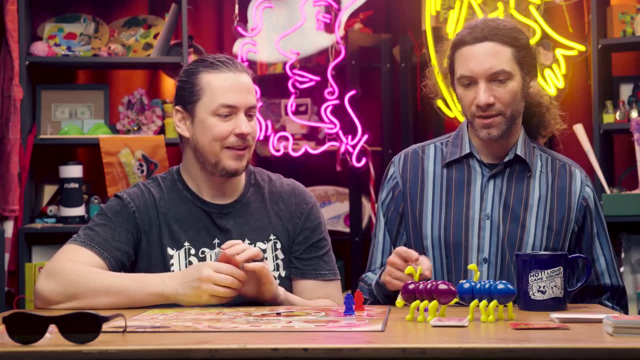 Okay, cool. Let's say, if you get Mr T, you lose automatically because he just beats the. So let's spin our spinner. I love it. Pimento cheese, Pimento cheese. Does that mean farmer's fate? Oh, I think that's farmer's fate. Banks raise prime rate, Pay 10% of outstanding loan balance as additional interest. I got it. Go to the nearest cash register. Oh, that one's good, That one's good. You owe the bank $1,000. And you have to select. 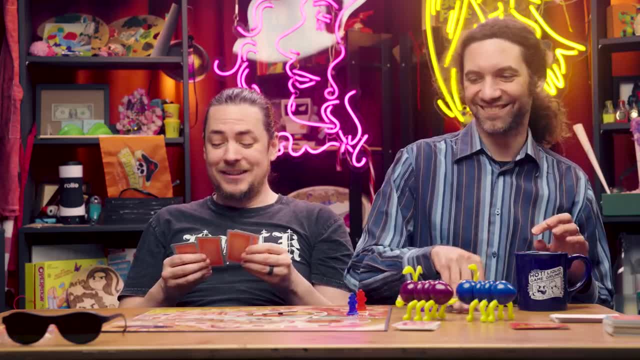 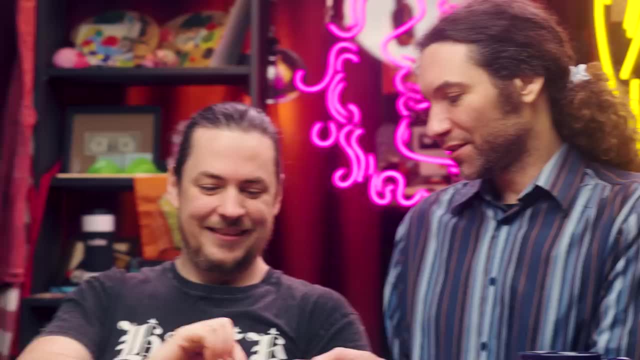